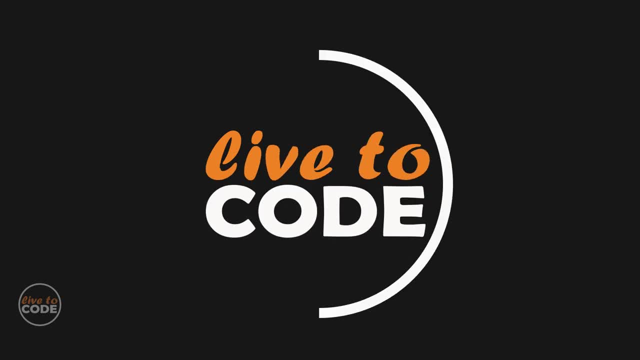 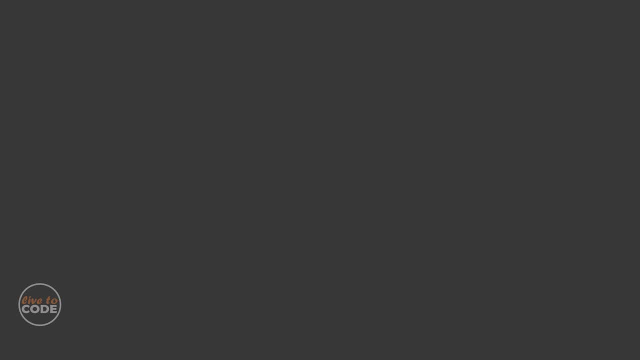 In this video we are going to see about recursion in detail. Let's take a classic example- Fibonacci- for recursion analysis. Each number in the Fibonacci series is the sum of two preceding numbers. If we add 1 and 1, we will get 2.. 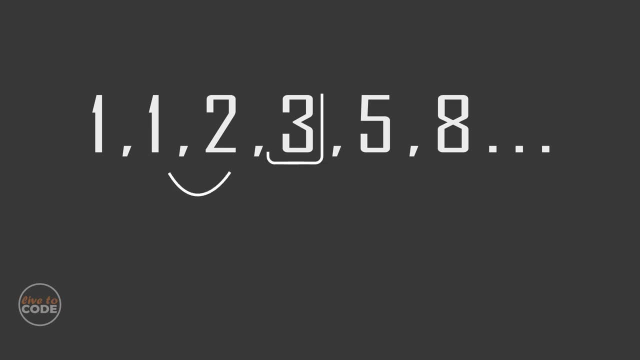 If we add 1 and 2, we will get 3.. If we add 2 and 3, we will get 5. And so on. Let's see the pseudocode for Fibonacci series for better understanding. This is the base condition. 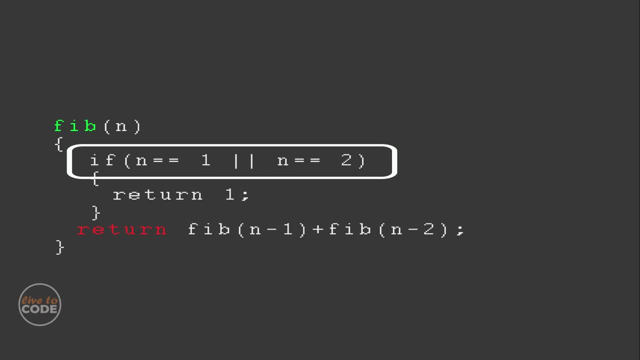 When n value comes into the function- 1 or 2, then Fib function will return 1.. This is the recursion call. Recursion means a function will be called by a function. Here Fib function is called by itself. When the base condition fails, recursion call will be happen. 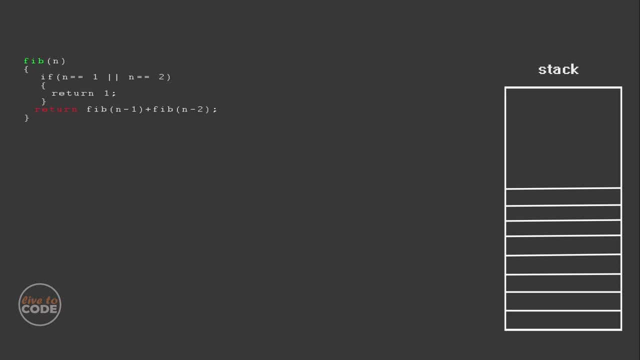 This is stack. Stack will track all the function calls. Let's see them elaborately. Our program will start from main function. Main function calls the Fib function with n value 5 and main function will be pushed into the stack Fib function with n value 5.. 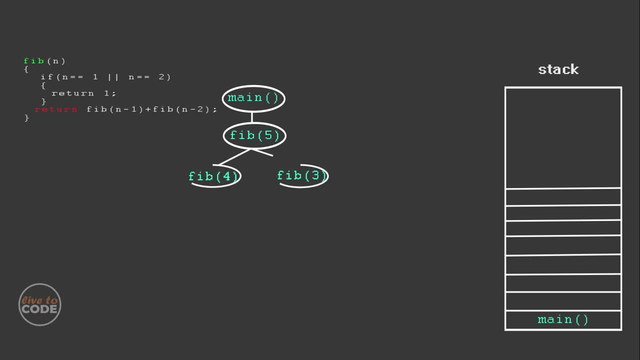 Fib function with n value 5.. Fib function with n value 5 will be called itself with n value 4 and 3.. So Fib of 5 will be pushed into the stack. Fib function with value 4 will call itself with value 3 and 2.. 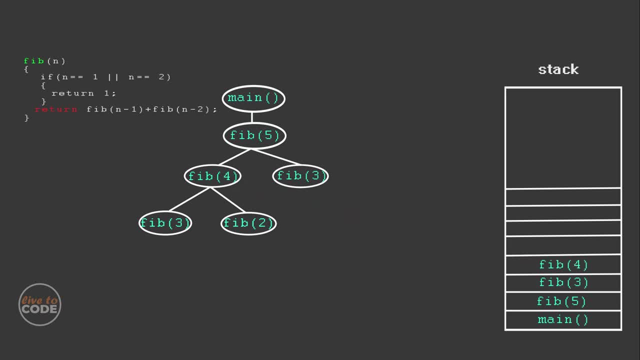 So Fib of 3 and Fib of 4 will be pushed into the stack. Fib function with value 3 will call itself with values Fib of 2 and Fib of 1.. So Fib of 2 will pushed into the stack and Fib of 3 also pushed into the stack. 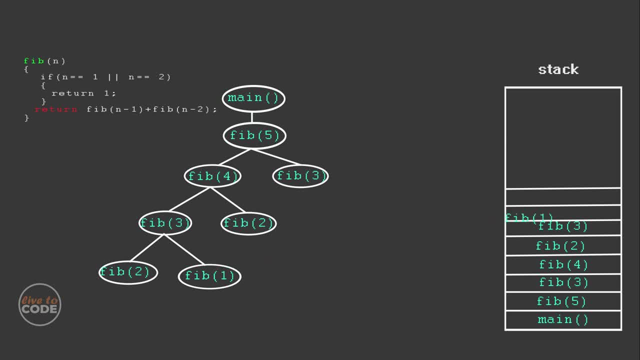 Now Fib of 2 will be called itself with n value 4 and 3. will be called itself and fib of 1 will be pushed into the stack As per our base condition. fib of 2 will return 1.. Then fib of 1 is popped out from the stack and call the function with n value 1.. 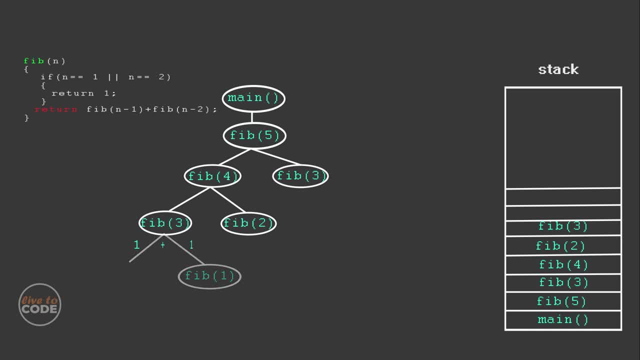 As per our base condition, fib of 1 will return 1.. After that, fib of 3 will be popped out from the stack and returns 2 to the previous call. Now fib of 2 will be popped out from the stack and call the function with n value 2.. As per our base condition, if n value is 2,,